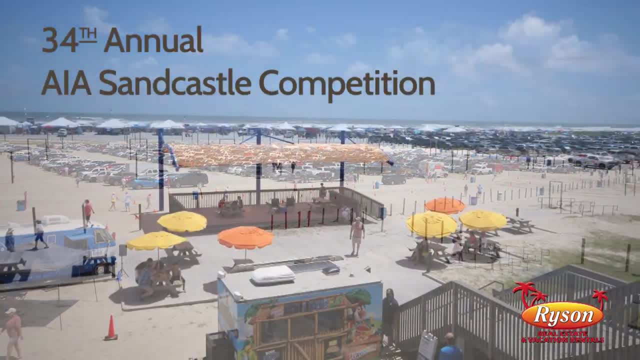 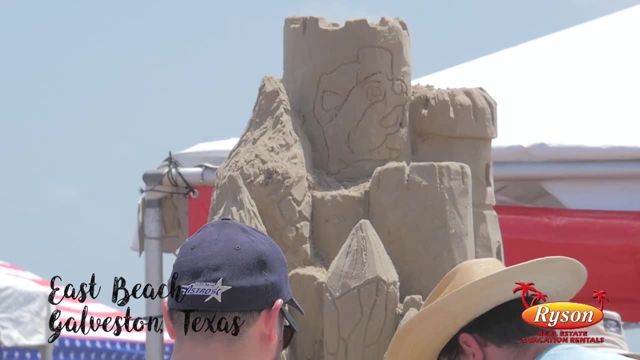 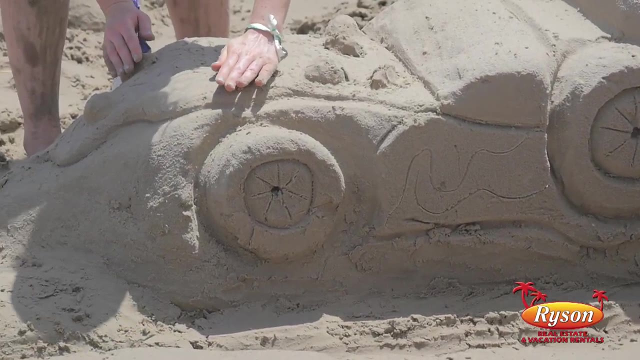 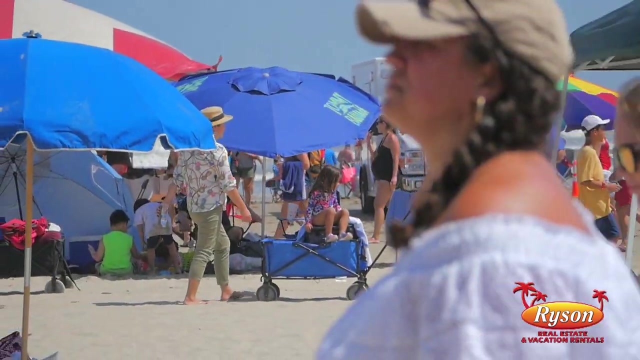 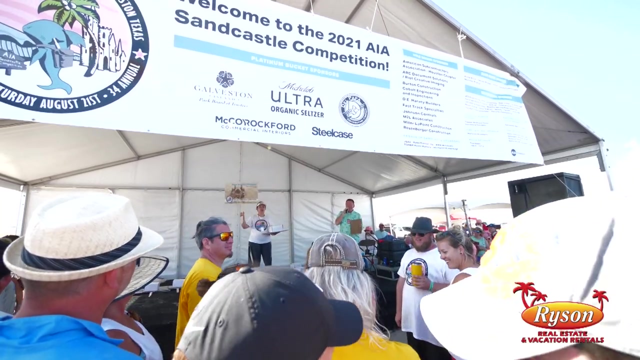 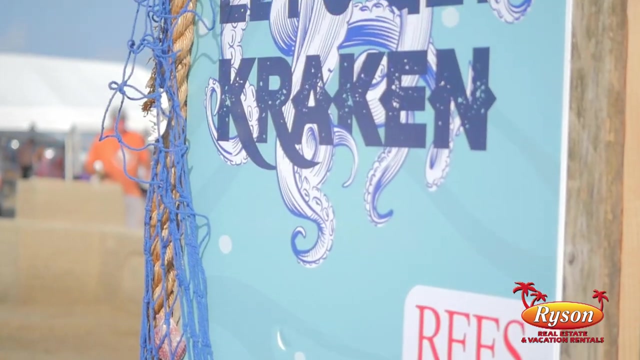 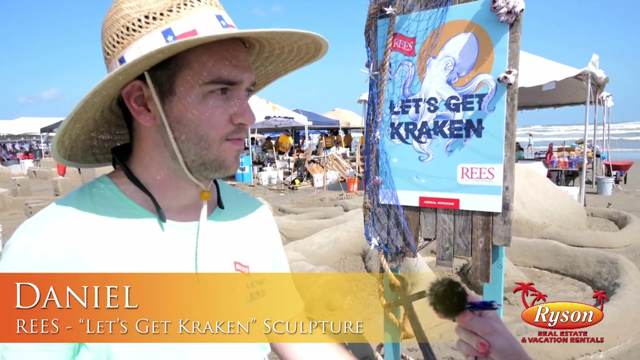 Animal Kingdom goes to site number 24, Reese. So I'm from Dallas, Texas. Our company is branching out in the Houston area. We have a lot of clients in Houston and we're working on our Houston office right now For our first time out. I think we got a lot of votes. 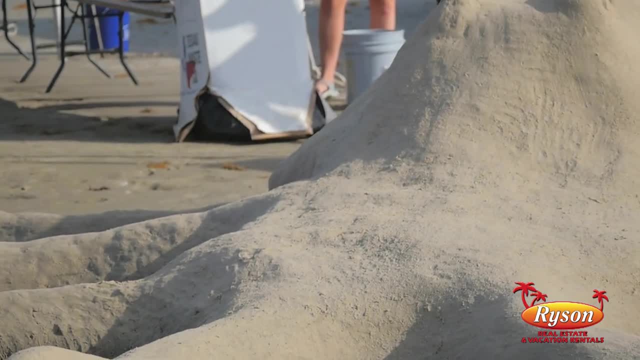 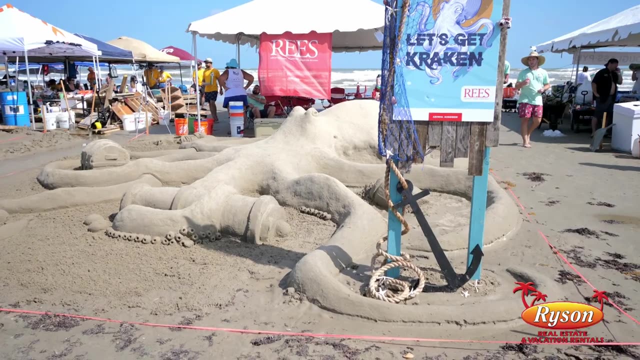 for People's Choice and we had a lot of fun doing it. It's been a great crowd, Everybody coming out has been amazing, So I've had a lot of fun. So we were really thinking: what can we come out and do our first year doing this? 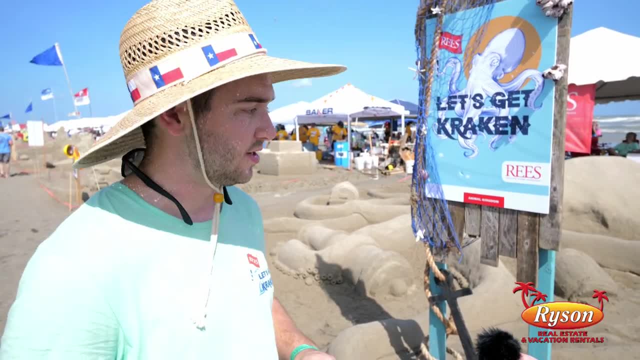 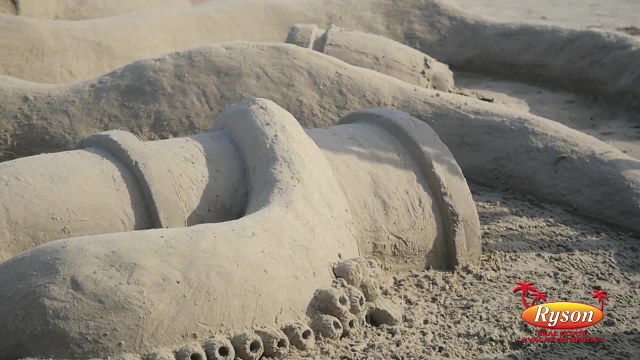 and be successful and kind of make an impact, get the crowd's attention. So we did something that was organic, that it didn't have to be perfect. It could have some lumps and bumps, because an octopus or a kraken would have lumps and bumps. 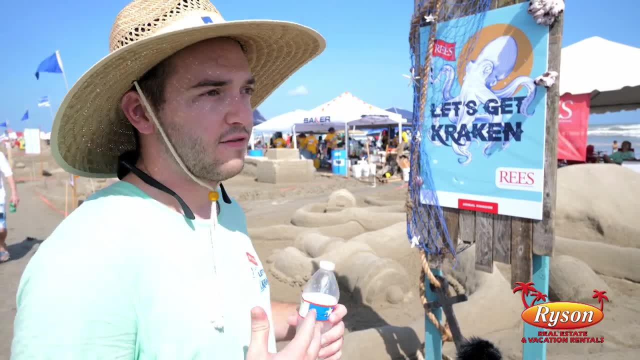 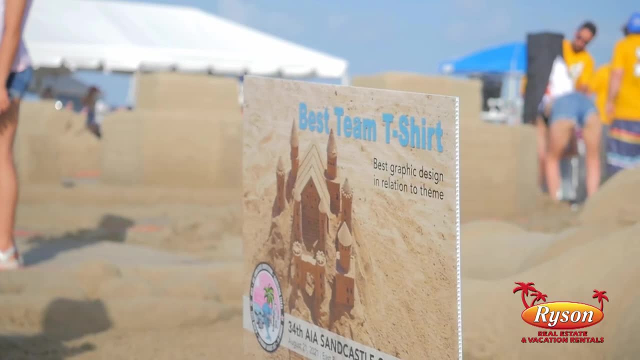 So hopefully we weren't going to get critiqued as hard if our craftsmanship wasn't as good- Something we could do and be successful at. So we didn't use any formwork, We kind of sculpted it all out of the pile that we were given. 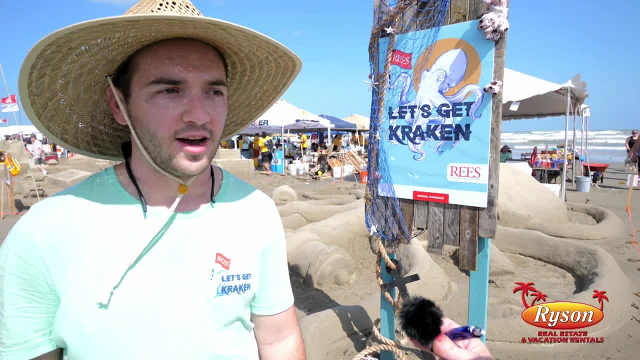 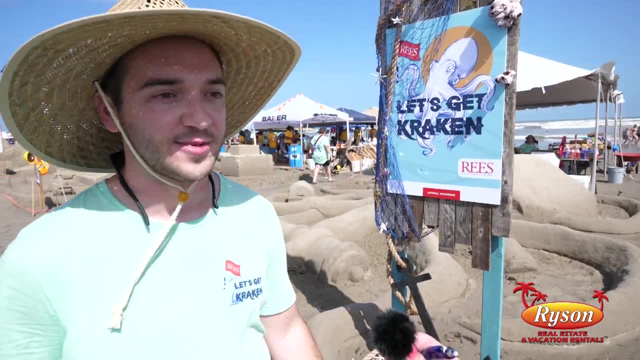 We started at about 7.30.. I think we were done by about 2 o'clock. Don't waste your time with formwork. It's a lot easier if you just come out here and try to sculpt something more organic. It's really hard to get these clean edges. 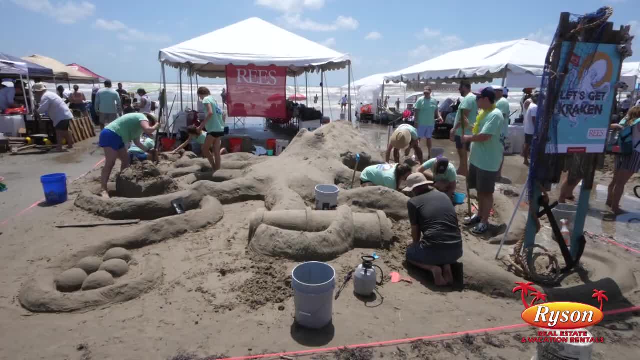 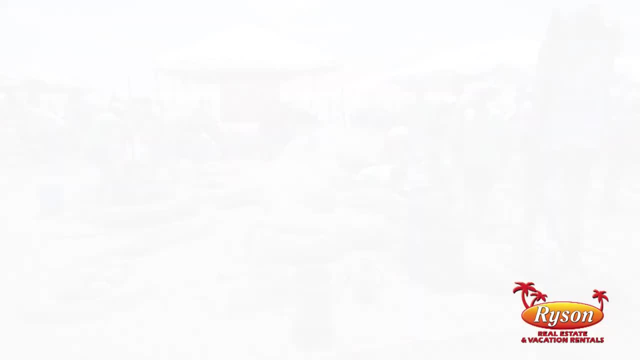 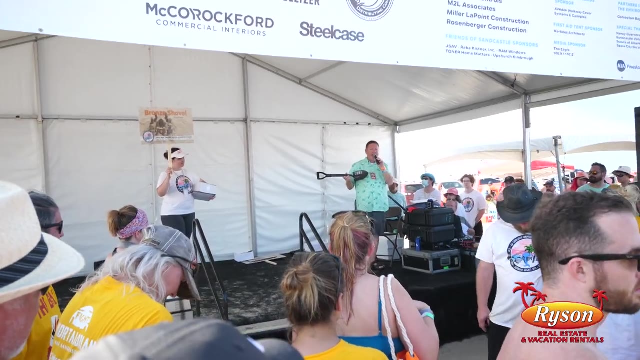 and orthogonal angles where things meet up. So yeah, just come out here and practice too. We practiced last night beforehand, so practice helps. The Bronze Shovel Award this year, Woo Woo, Goes to site number 10, Kirksey. 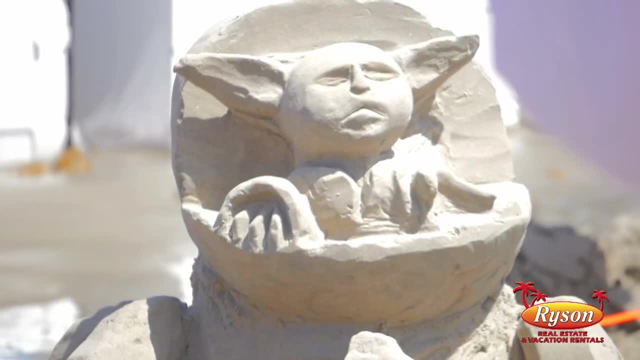 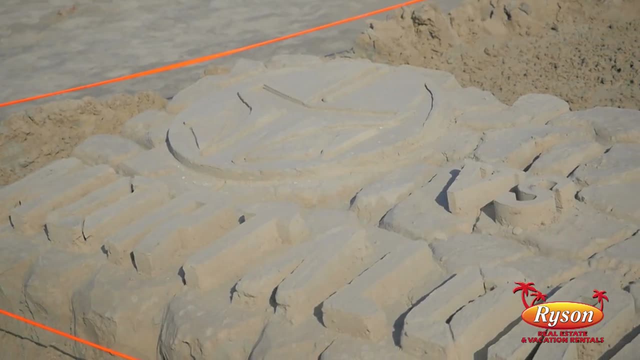 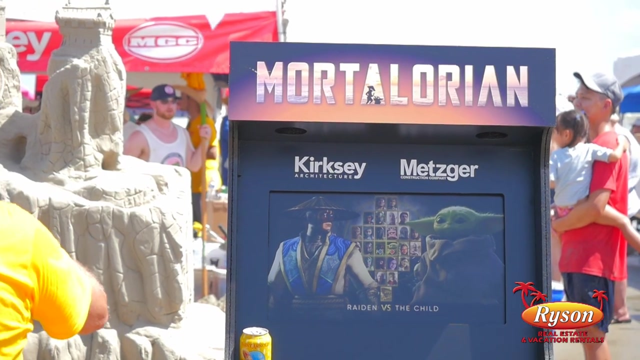 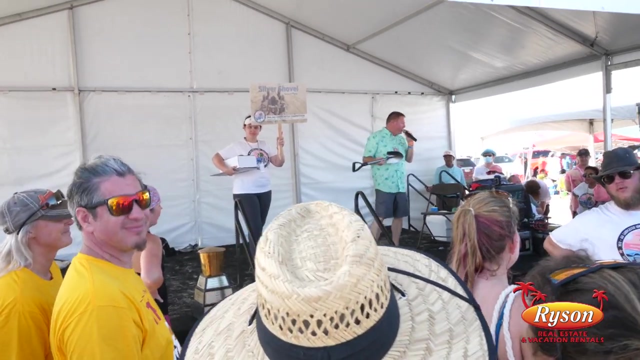 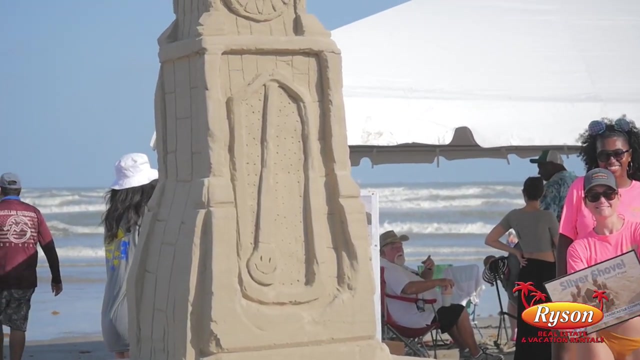 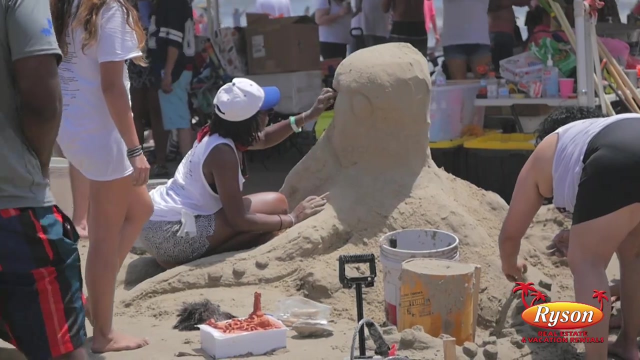 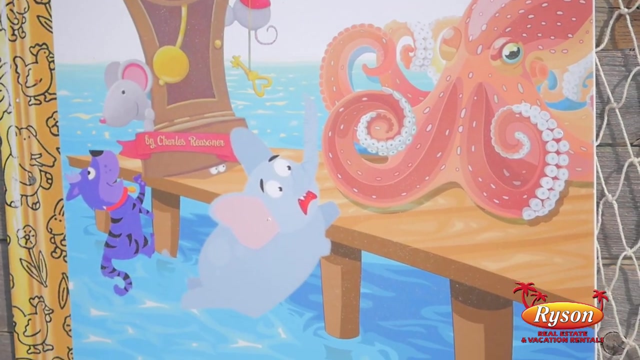 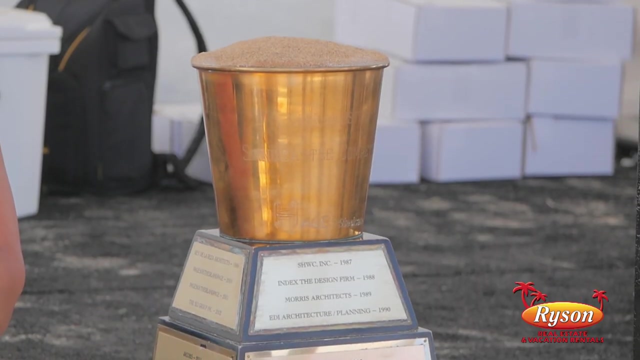 Woo Best team signage For the Silver Shovel Award. second place prize this year goes to site number 13, PGAL Woo Woo. And now we have Rusty here to help us award the Golden Bucket first place for the next year. 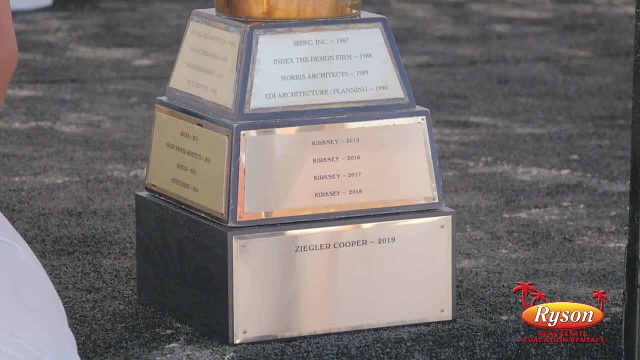 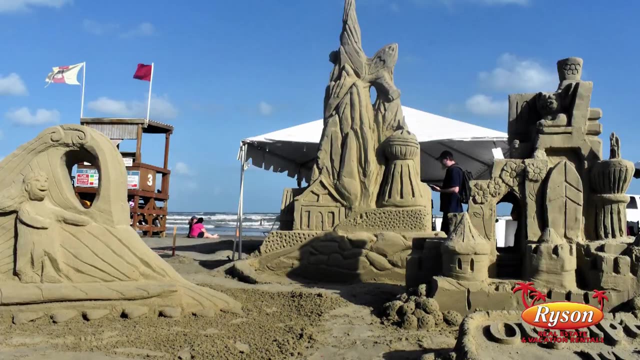 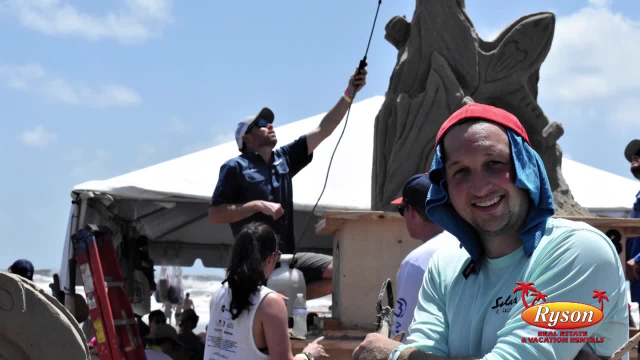 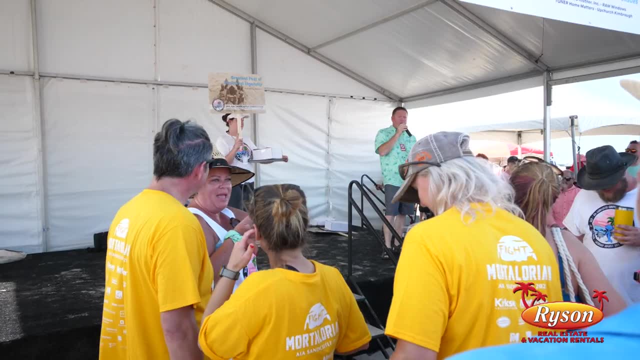 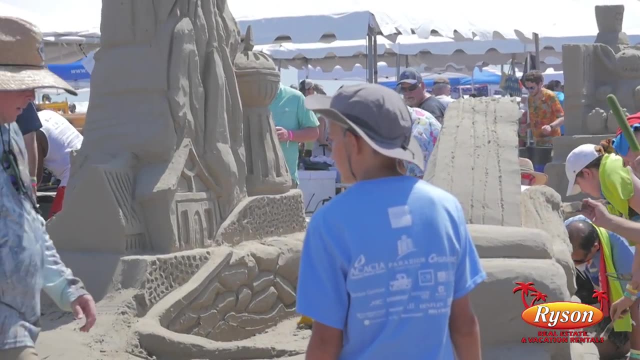 Now, as architects, engineers, other design professionals, we all go for best structural ingenuity. That one goes to number 14, Ziegler, Cooper. And now for the part all of you people signing all of those papers worked so hard for. 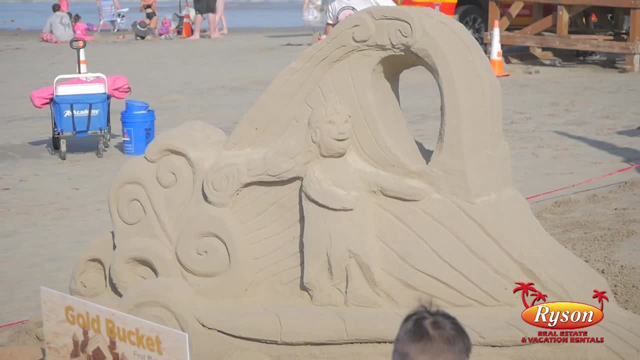 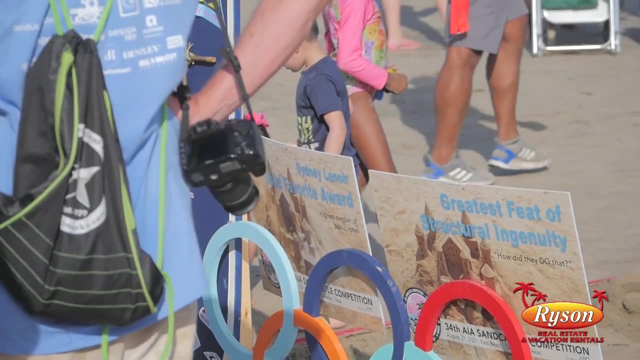 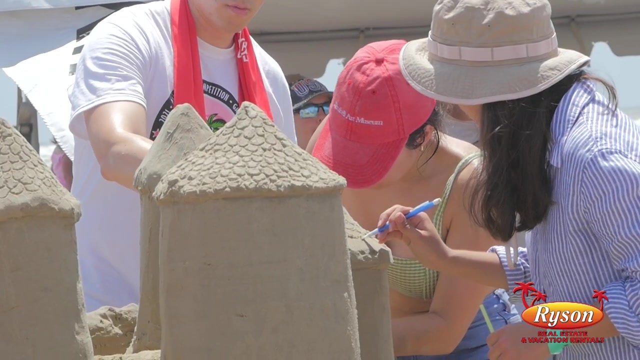 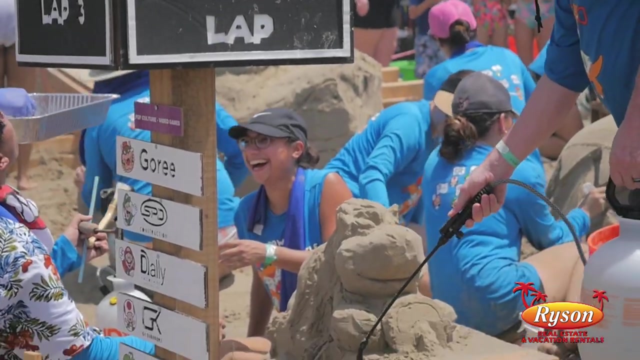 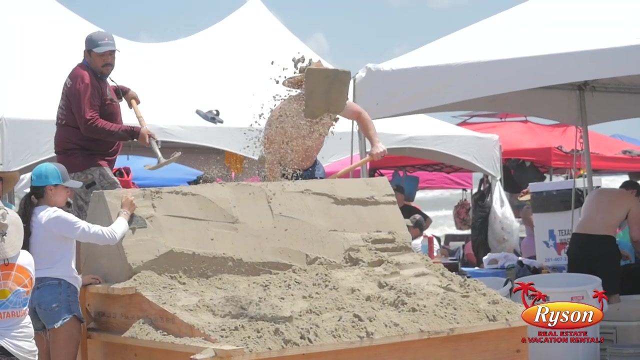 The Sidney Lenore Public Favorite Award goes to Ziegler Cooper, sight number 14!. The Sidney Lenore Public Favorite Award goes to Ziegler Cooper, sight number 14!. And now for the part. all of you people signing all of those papers worked so hard for. 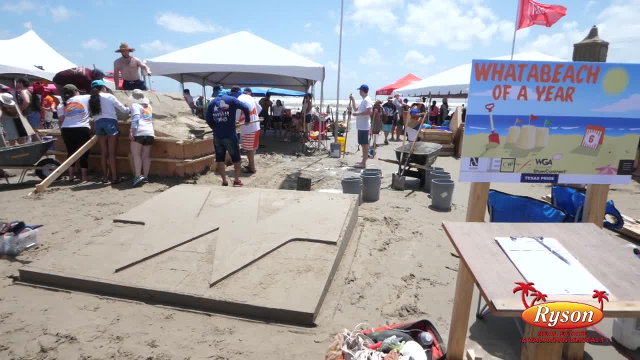 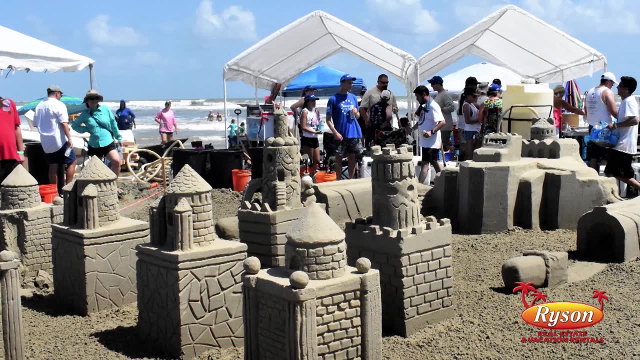 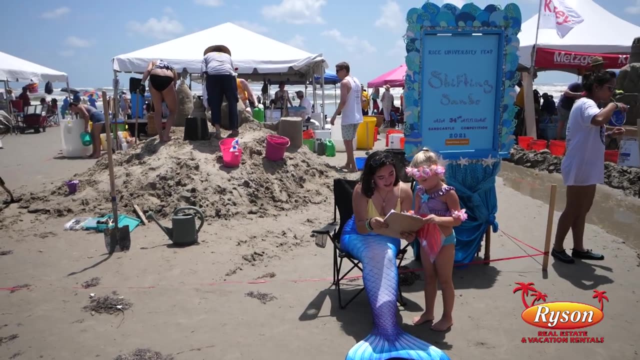 The Sidney Lenore Public Favorite Award goes to Ziegler Cooper, sight number 14!. Now, as architects, engineers, other designers, we all go for best structural ingenuity. The Sidney Lenore Public Favorite Award goes to Ziegler Cooper, sight number 14!. 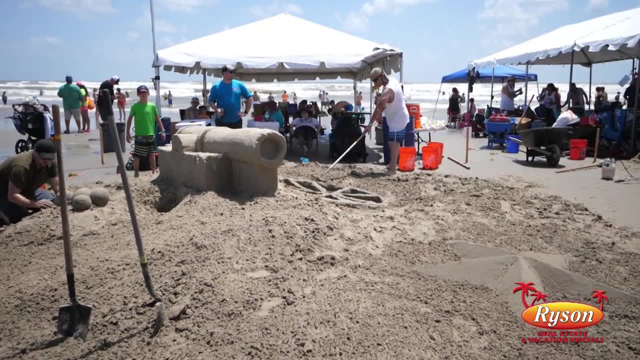 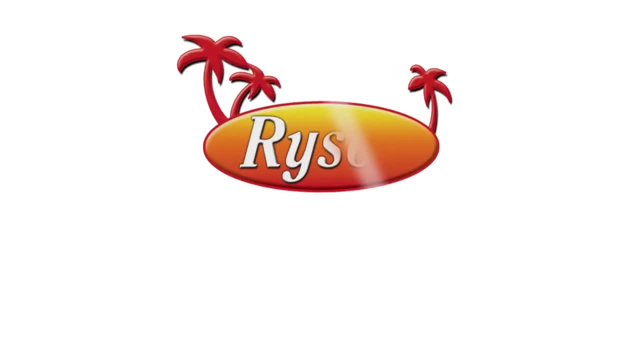 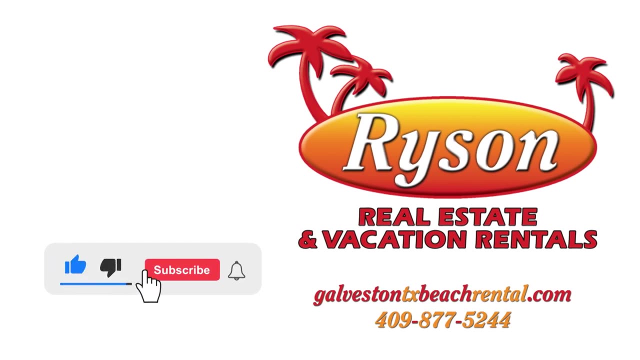 I'll see you next time.